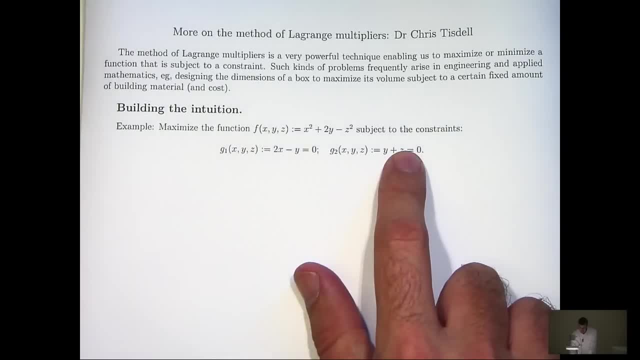 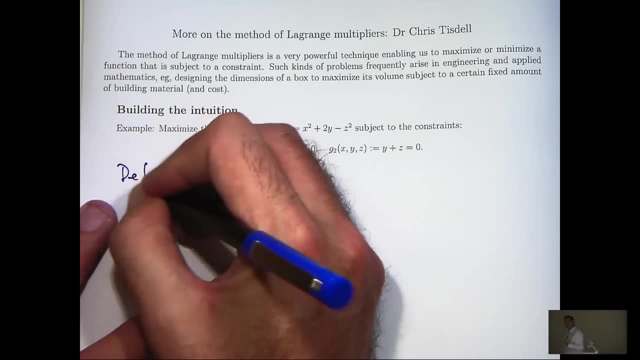 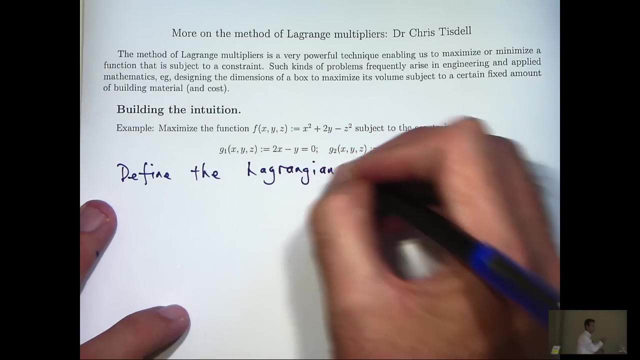 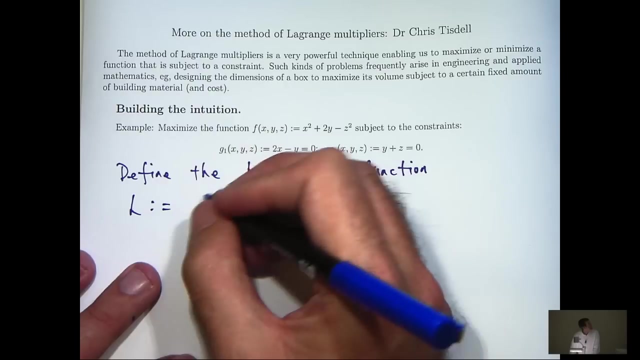 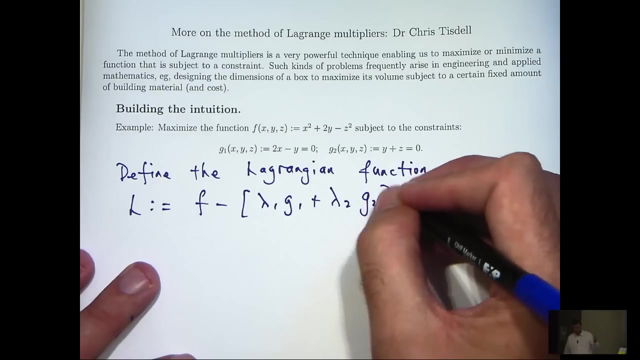 asked to maximise this function subject to two constraints. Okay, so we're going to define the so-called Lagrangian function, which we denote by L, and it's defined in the following way: Now, the lambda one and the lambda two are the. 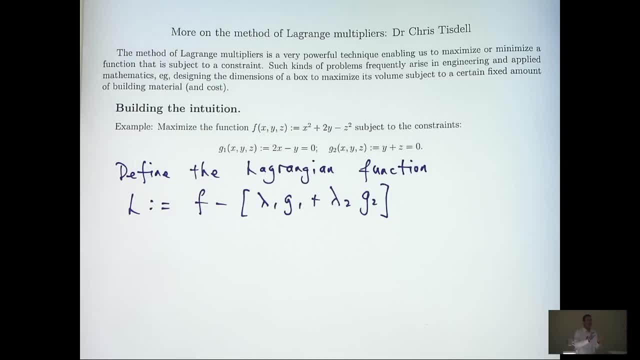 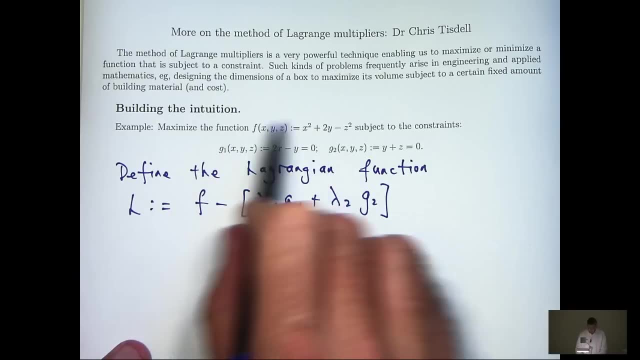 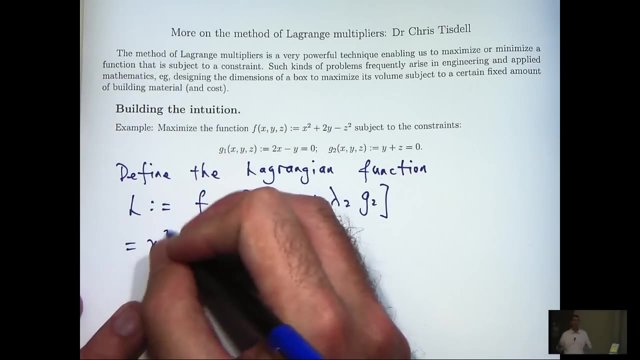 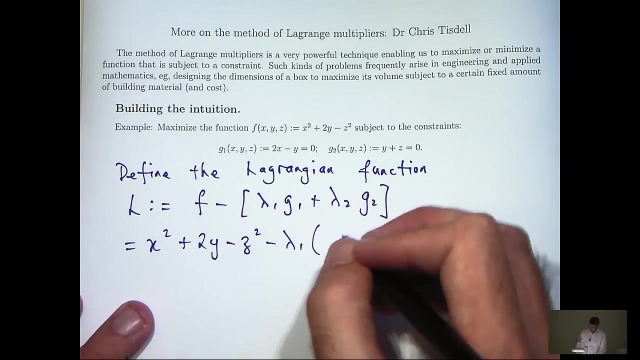 same. So the lambda one and the lambda two are the same. So the lambda one and the lambda two are the so-called Lagrange multipliers for this problem. Now, they're just numbers, So if F and G1 and G2 are defined in the above way, let's actually write them out in full. 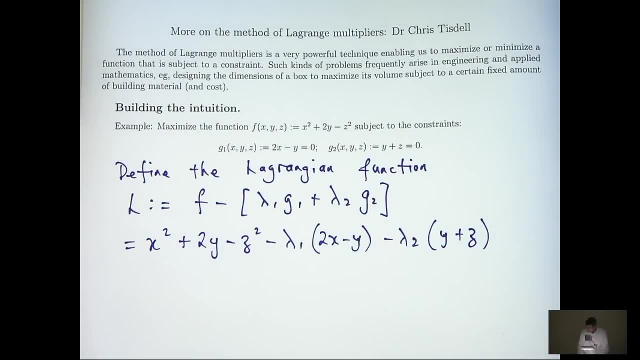 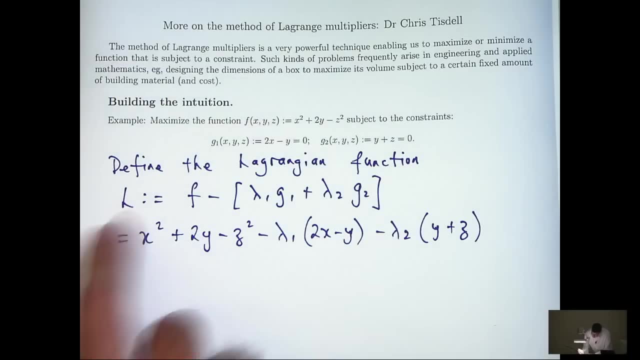 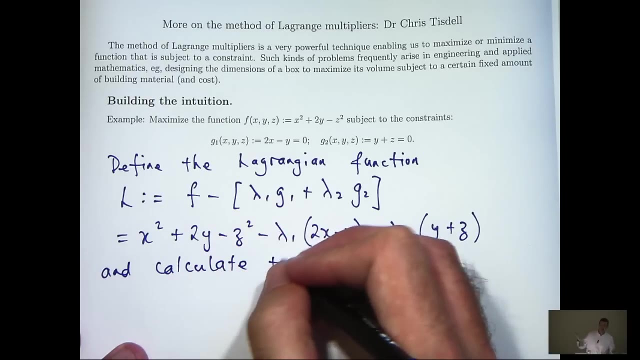 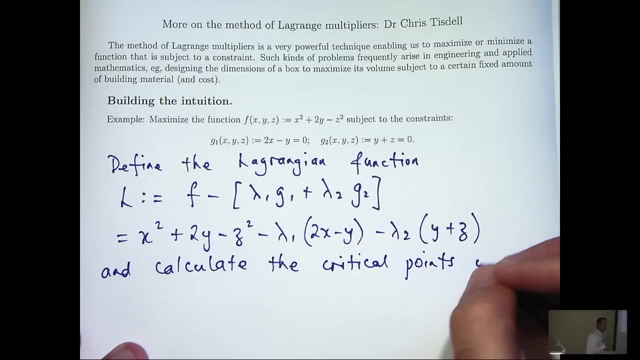 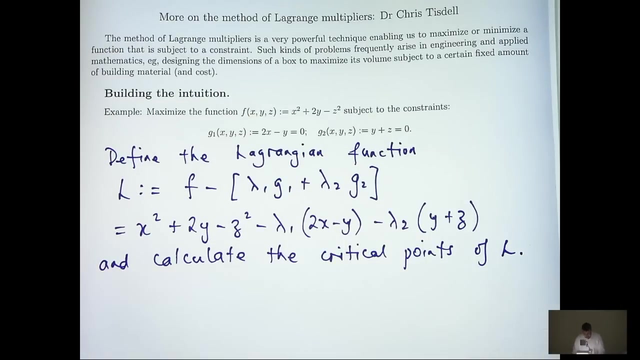 Okay, and what the method of Lagrange multipliers involves is actually calculating the critical points of L. Now we know from calculus that you've got to have some kind of L in order to calculate. And to calculate the critical points, then what we do is calculate the partial derivatives. 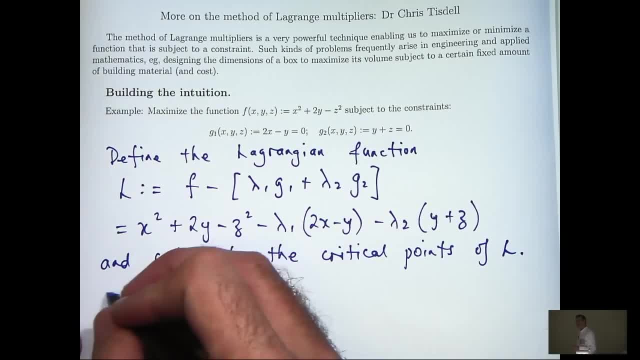 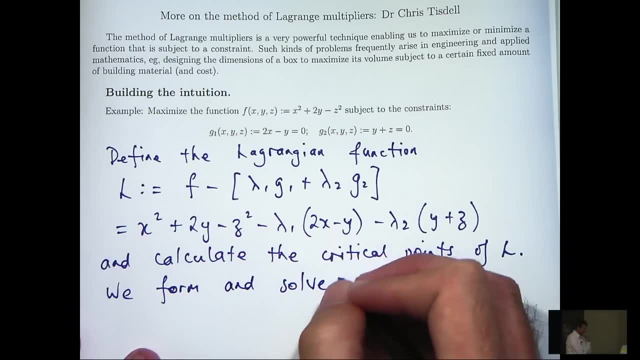 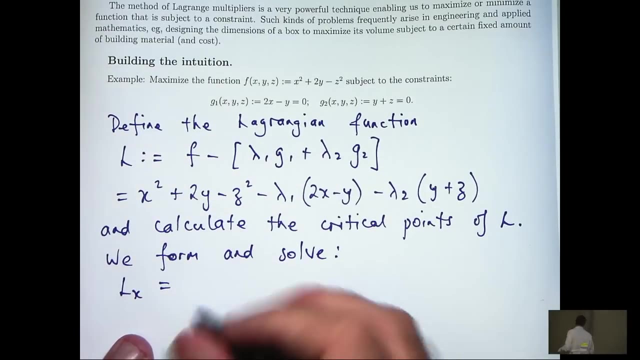 of L and set them equal to zero and solve. So let's form the partial derivatives of L, set them equal to zero and then solve the resulting equations. Now by a subscript, here I mean dL, dx. the partial derivative of L with respect to x. 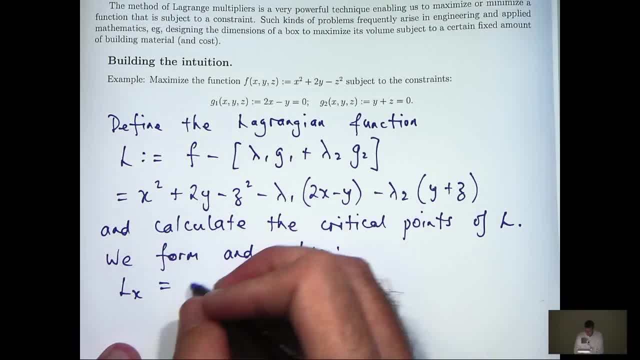 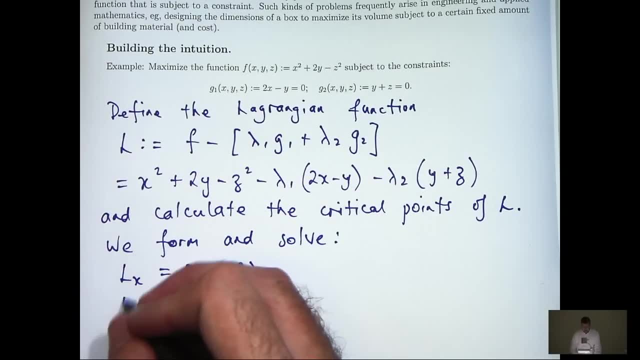 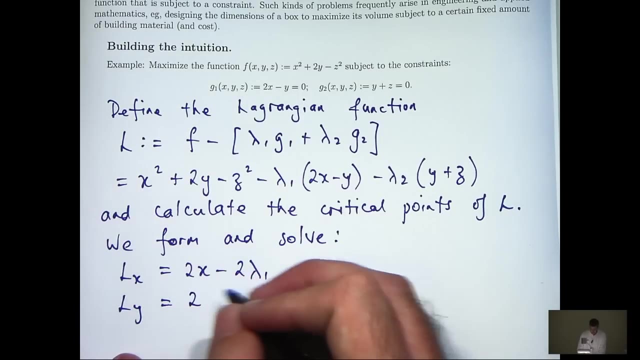 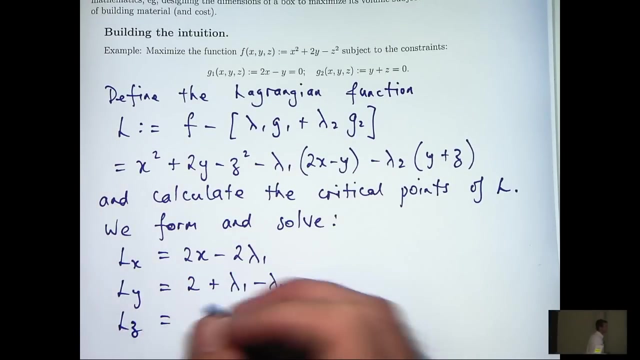 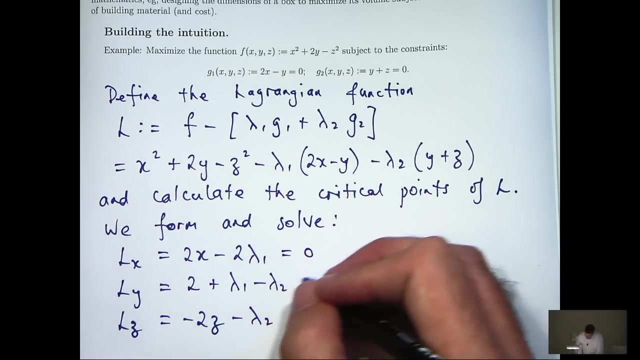 So we go up here, differentiate with respect to x, holding everything else constant, and we'll get something like this: Similarly, L sub y, partial derivative of L with respect to y. L sub z. Okay, To find the critical points, we set these equal to zero. 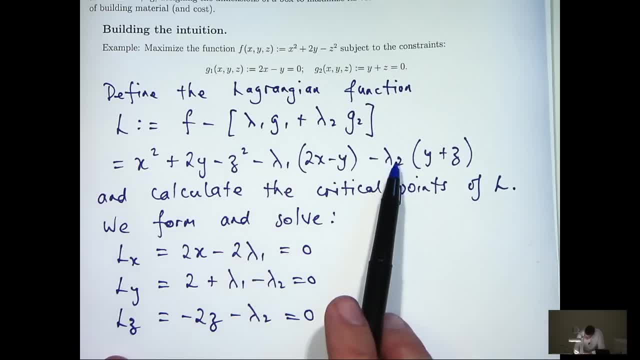 Now you may be thinking: well, hang on, L also depends on lambda 1 and lambda 2.. What about the partial derivatives with respect to lambda 1 and lambda 2?? Well, actually, if we calculate those partial derivatives and set them equal to zero, they're 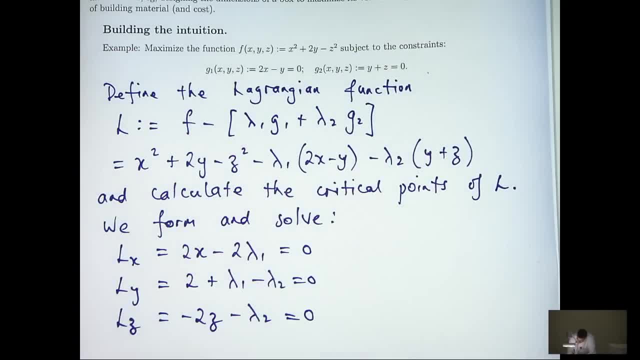 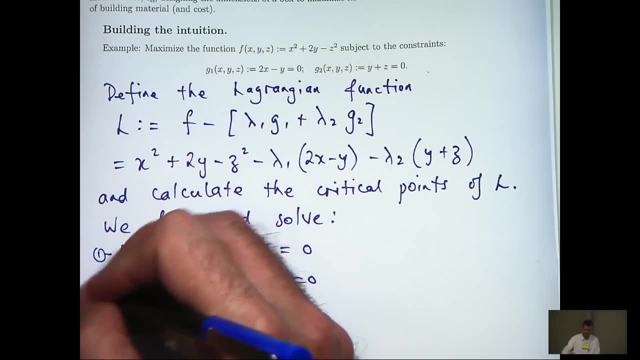 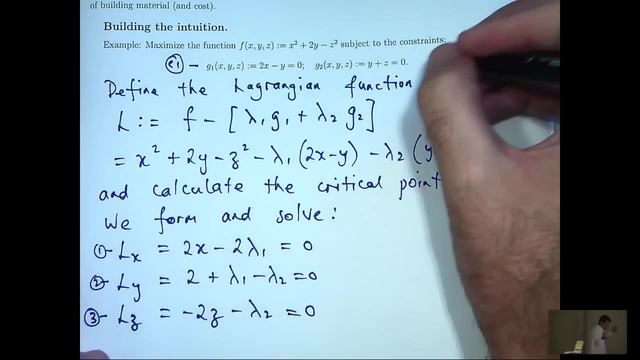 actually the constraint equations, So I don't really need to do those calculations, Okay. Well, I'm going to number these equations Okay, Because I'll refer back to them, and I'm going to number these as C1 and C2, constraint. 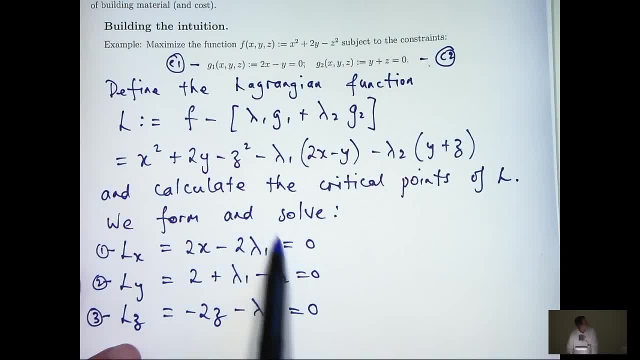 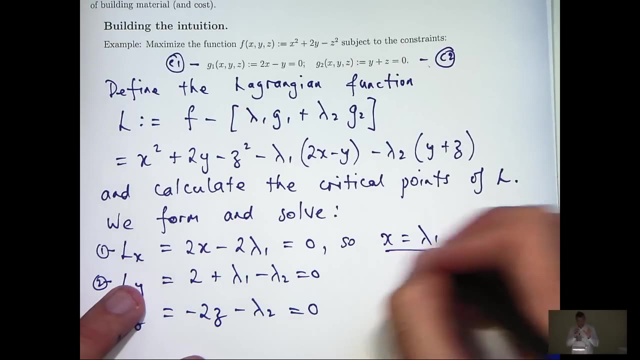 1 and constraint 2.. So what I would like to do is solve the five equations for x, y, z, lambda 1, and lambda 2.. Okay, So I can rearrange first to get x equals lambda 1 up here and I can rearrange down here to 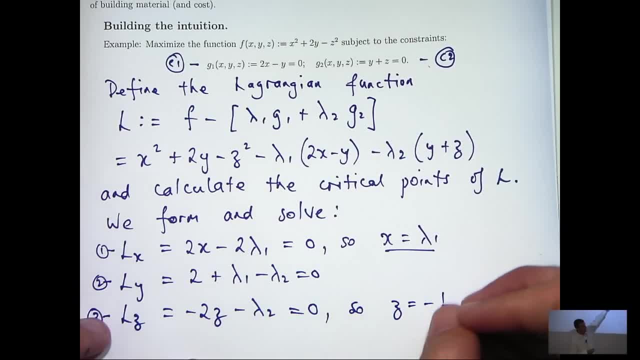 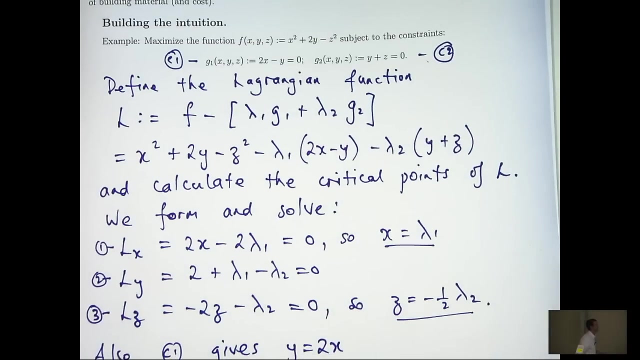 get z equals minus 1 half lambda 2.. Now I can rearrange C1 to get y equals 2x. So what I'm trying to do now is just simplify everything and see if I can come up with x, y and z. 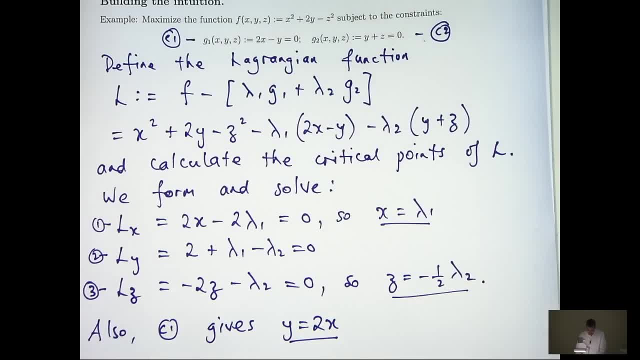 Okay, Okay, Lambda 1 and lambda 2.. Okay, Well, if I look at these two, I can immediately form a relationship between y and lambda 1.. y will equal 2 lambda 1.. Okay, And now I can form. if I look at this: y equals lambda. 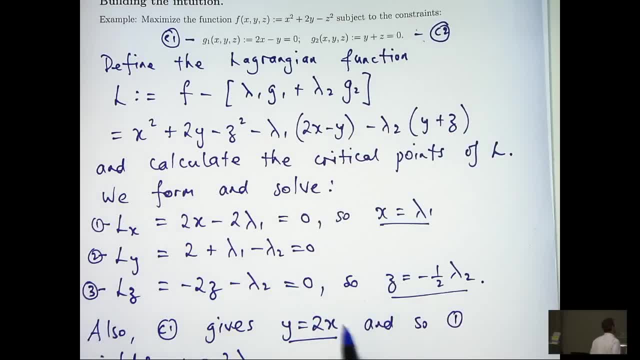 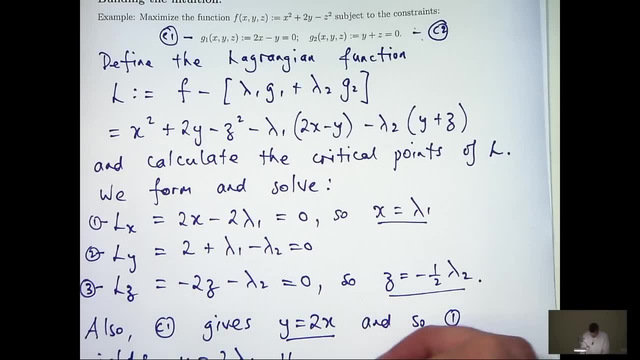 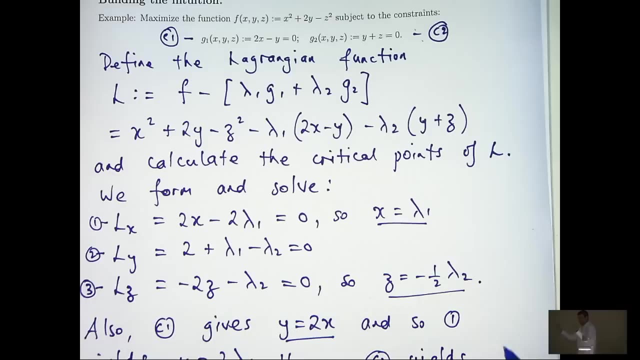 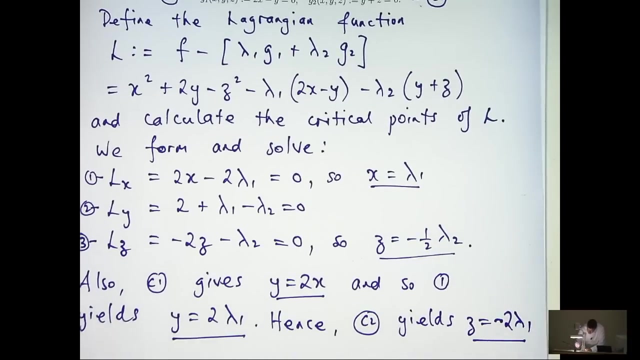 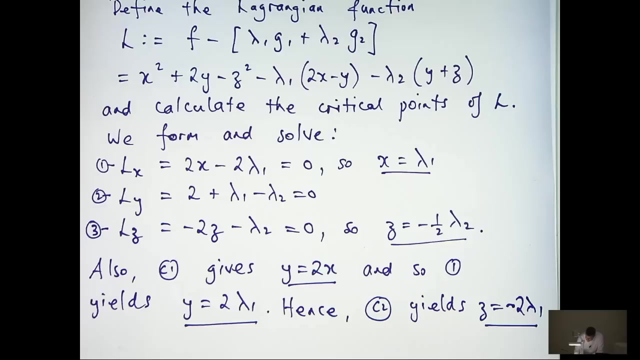 Sorry, Y equals 2 lambda 1 and C2, then I can form a relationship between z and lambda 1.. So z will equal negative 2 lambda 1.. Okay, Okay, Okay, Okay, Okay, Okay, Okay. well, let's look now at these two underlined expressions here. 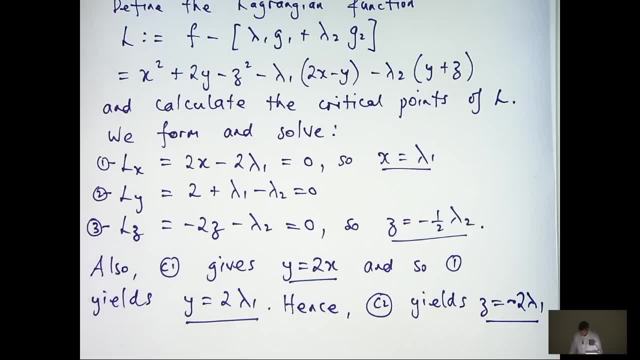 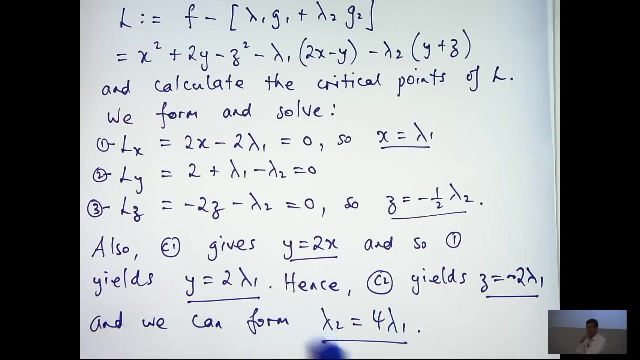 I can form a relationship between lambda 1 and lambda 2.. If I look at this, just substitute in here and rearrange, I'll get lambda 2 equals 4 lambda 1.. Now I can take that and substitute it in here for lambda 2.. 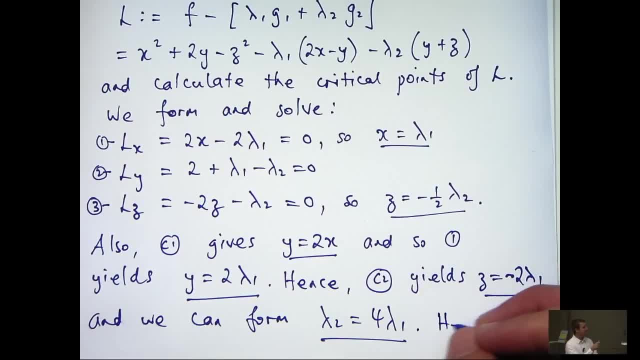 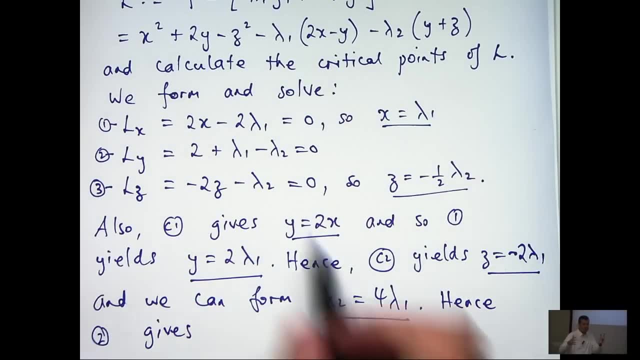 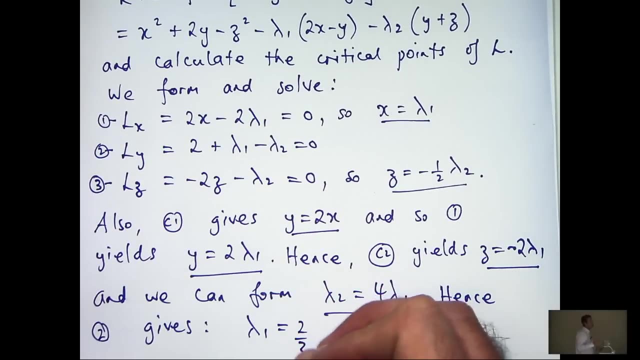 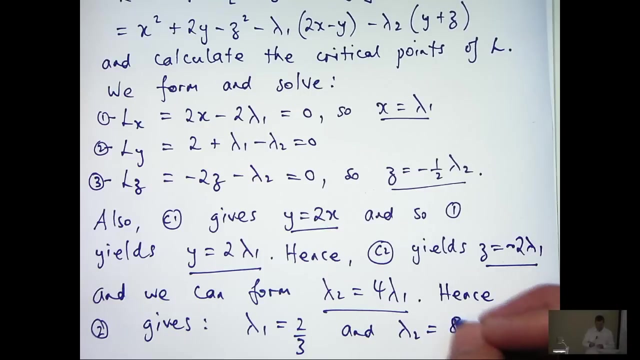 So if I substitute in there, I'm going to get lambda 1 equals 2 3rds, and lambda 2 equals 4, 2 3rds. OK, 2 equals 8 thirds. So this is the important information here that we're going to work with. 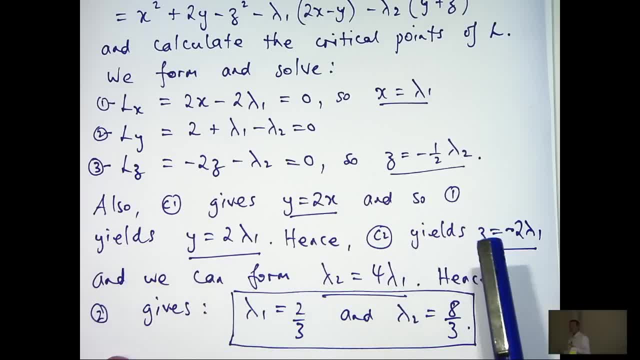 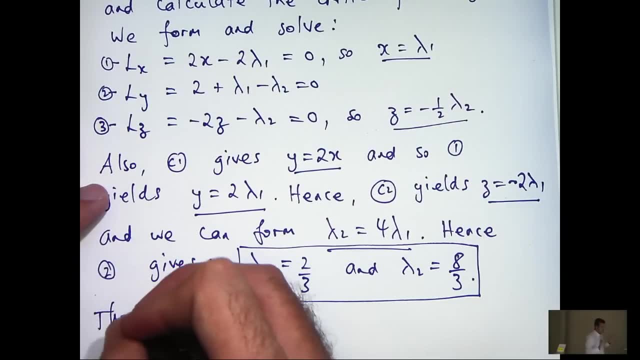 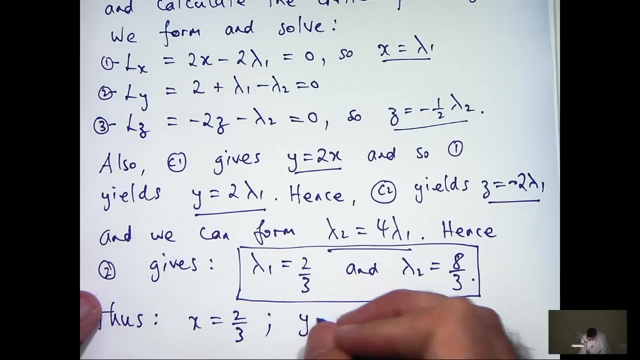 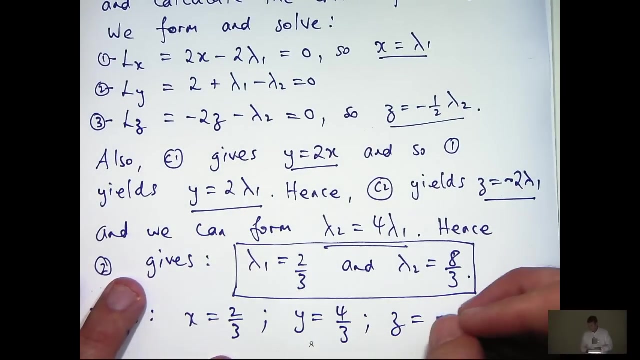 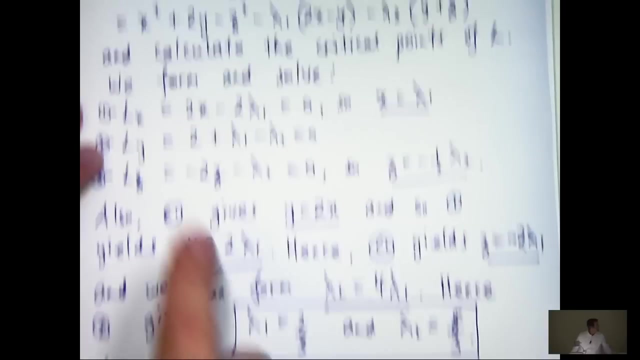 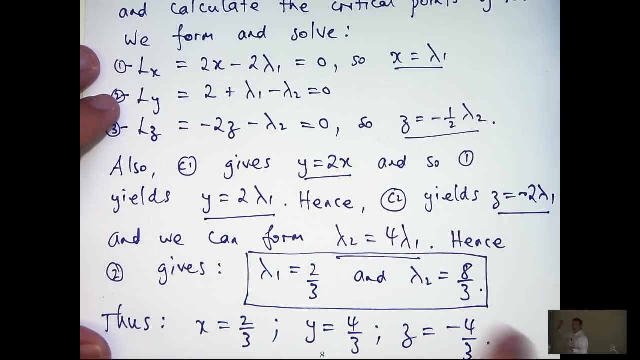 What I can do now is back, substitute and get x, y and z from these. So x will equal 2 thirds, y will equal 4 thirds and z will equal minus 4 thirds. So what information have we got there? Well, we know that our Lagrangian function has a critical point at these coordinates. 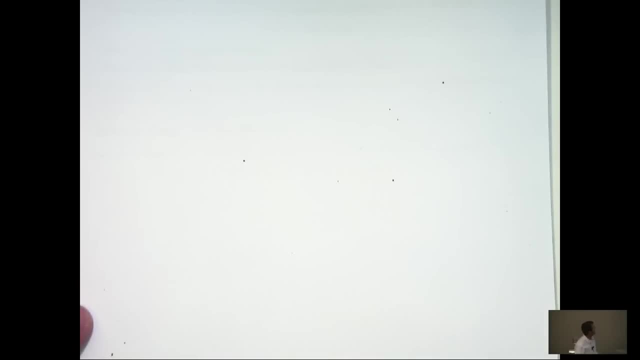 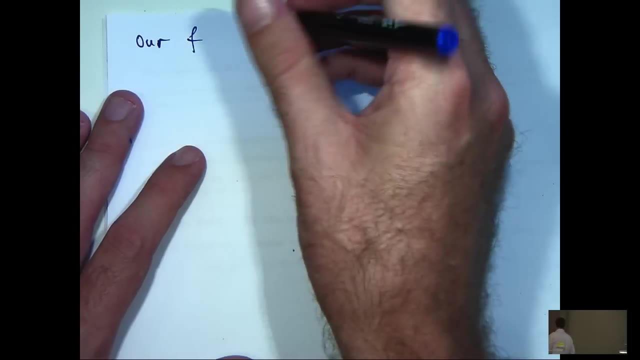 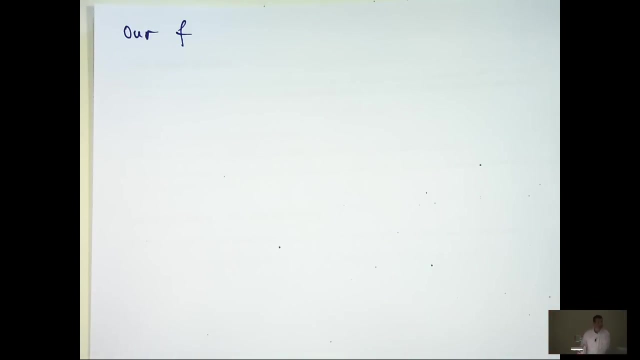 So let's do that. Let's make a conclusion Now. the method of Lagrange multipliers then says that f will have a maximum or minimum value at that point, And from the question we know that f is going to have a maximum. 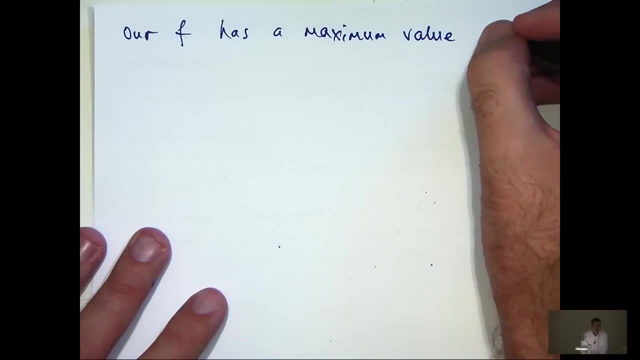 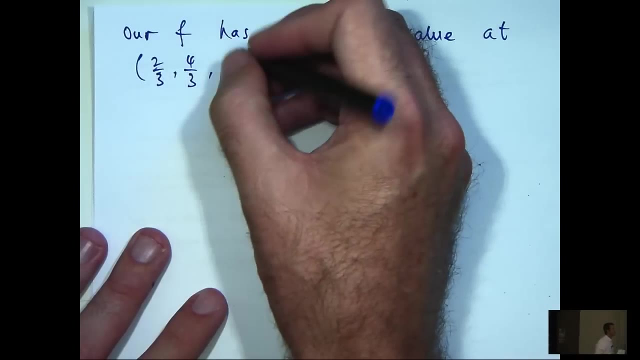 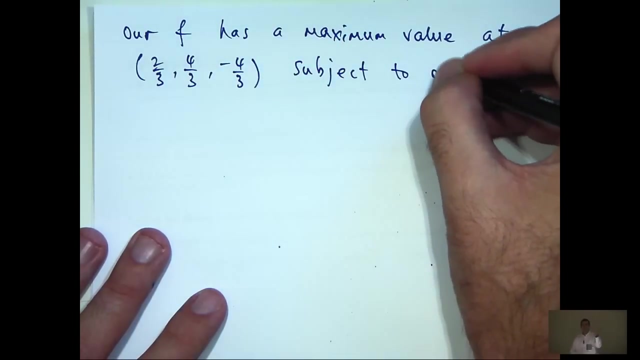 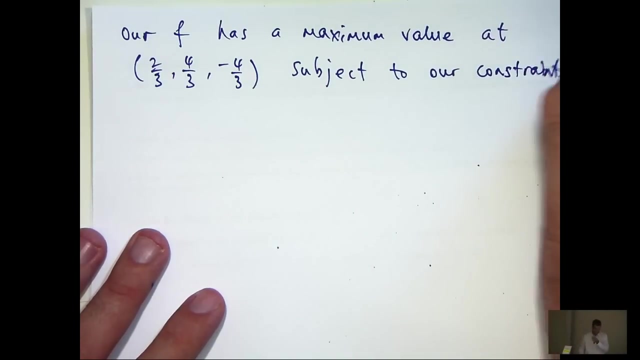 Let's say f is less than or equal to 0. And if f is less than or equal to 0, we know that f is going to have a maximum. Now, what is the maximum value of f? What is the value of f?